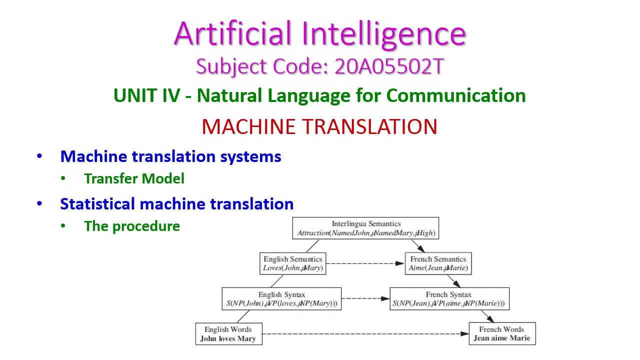 In this artificial intelligence class we will see the machine translation that will come under fourth unit, natural language for communication. So under this machine translation, two sub topics there. First one is machine translation system. Under this we will see transfer model and second one is statistical machine translation, and the procedure for machine translations are there. So here we will see the six steps to translate One language sentence. 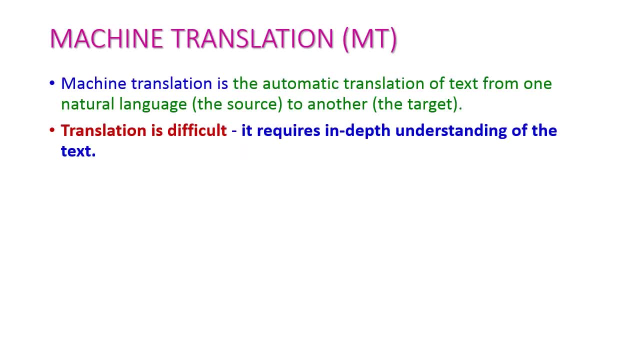 to another language sentence: Machine translation, which is otherwise called as MT. What is machine translation? It is an automatic translation of text from one natural language to another natural language, For example, translating the content from English language to Telugu language or Tamil language. It is very difficult process because 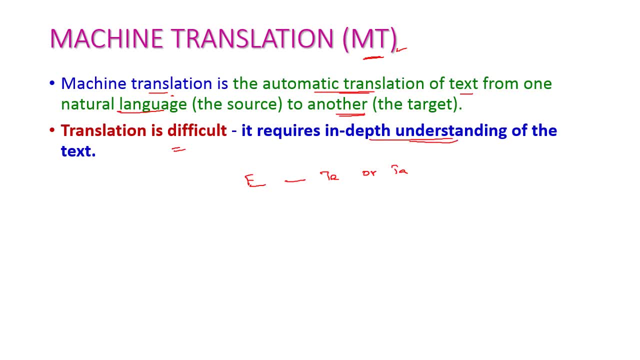 it requires in depth understanding of the text. Why means that grammar of Telugu language or Tamil language is entirely different from the grammar of English language. That is all. South Indian language grammar will be somewhat different from the English language grammar. So first we have to understand the concept. then only we can translate that concept into the target language. 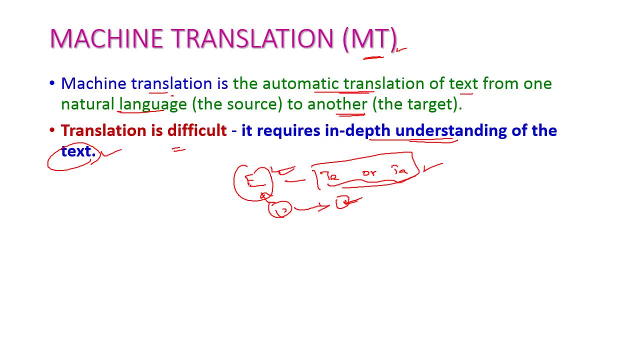 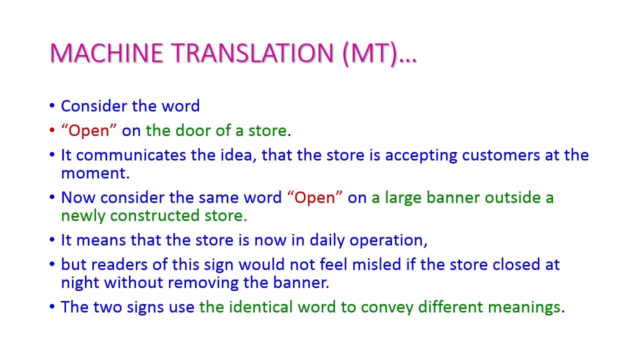 That is another natural language, So machine translation is somewhat difficult one. Let us see one example for this. Consider the word open. The open is in front of the door of a store. That means the store is accepting customer at the moment. That means previous day evening the store was closed and next day morning it. 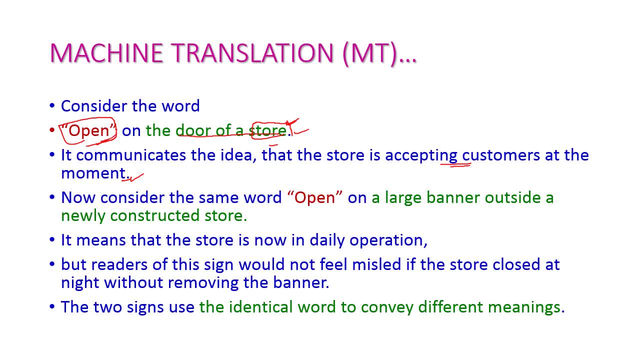 got opened. This is the meaning of this particular open. Now consider the same word open in front of a large banner outside a newly constructed store. So newly constructed store means it is not previously closed and today morning opened, because now only the store got inaugurated. 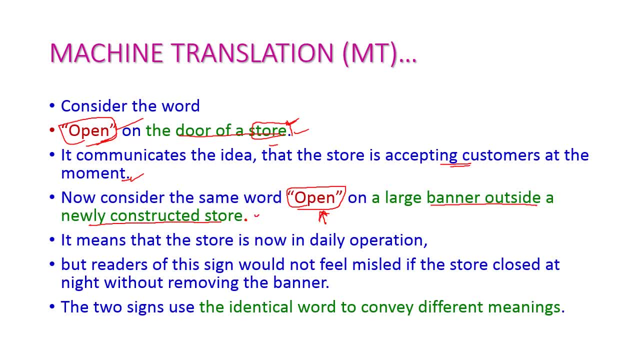 So from today onwards the store will come for functioning to accepting the customers. Hence this open and this open are entirely different. ok, So that before translating the content from one language to another language first we have to understand the concept first. 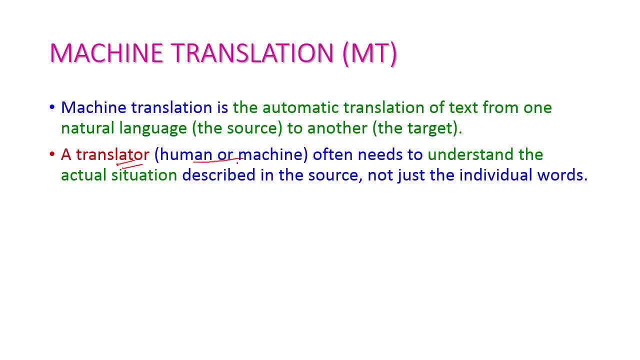 The translator. translator may be either human or machine. Machine needs to understand the actual situation described the source, not the individual words. If you translate word by word, you will not get the actual concept. So we have to understand the actual situation before translating the content. 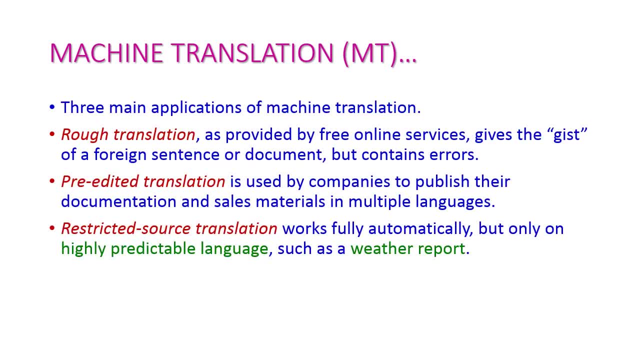 The applications of machine translation. Now let us see only three main applications. First one is rough translation and second one is pre-editor translation and third one is Japan. You can see… one is restricted source translation, Rough translation. Rough translation means the translations. 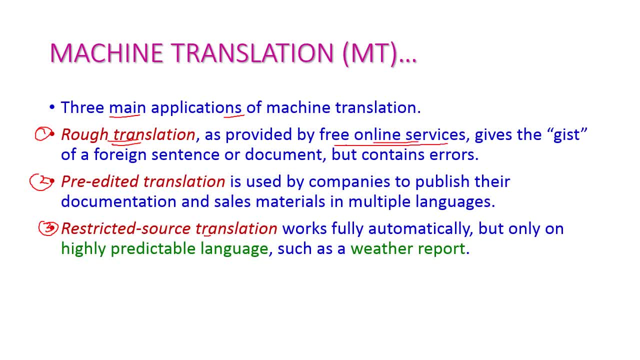 by using free online services. okay, Some of the free service providers are there. They will translate one language content to another language content. okay, But this contains errors, right? So this is called as rough translation And second one is pre-edited. 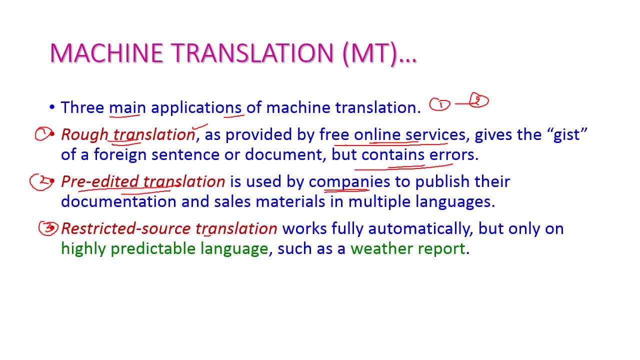 translation. These translations used by companies to publish their documents and sales materials in multiple languages. okay, So there is. there should not be any errors in this content, because those are very sensitive one. Hence they are using pre-editor translation. So 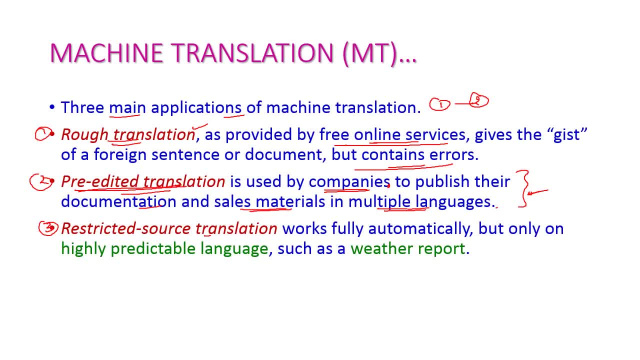 without any error, the translations will be taken place. And the third one is restricted source translation. okay, So this works fully automatically, fully automatically, But it only on highly predictable language. That means a very limited set of words or sentences are there, okay? For example, weather report. So weather report means it contains 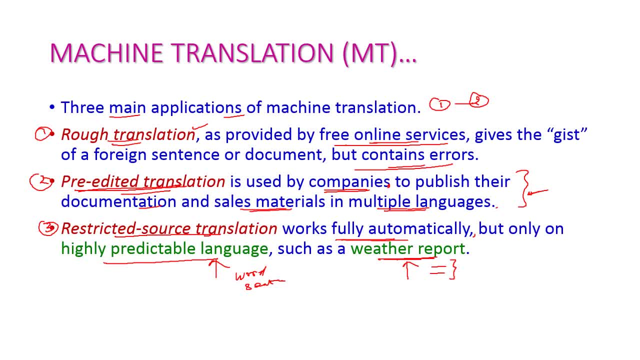 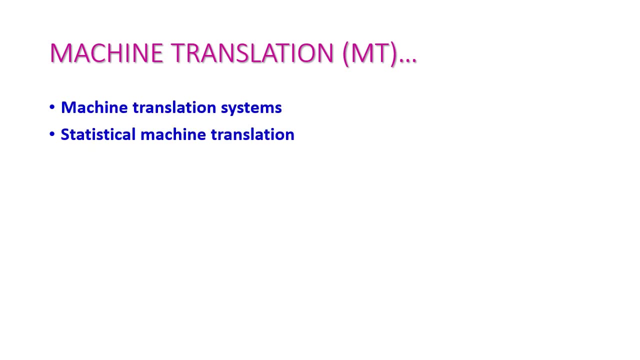 only limited set of words or limited set of sentences That will be suitable for all type of weathers. That means this type of translation will exclusive for a particular applications only. There are two subtopics in machine translation. First one is machine translation system and 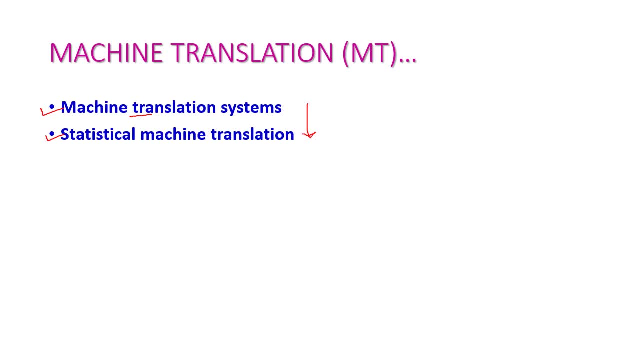 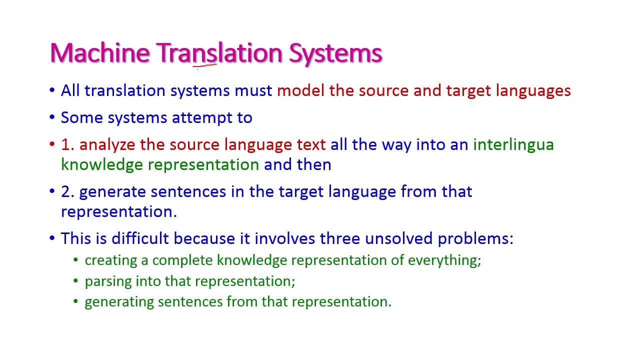 second one is statistical machine translation. Let us see all those things one by one, Machine translation systems. when come to machine translation system, all the translation system must model the source language and the target languages. okay, The system should learn both the source language and target language content. 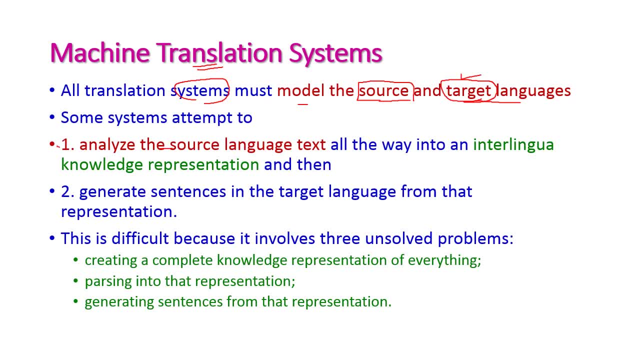 Okay, Some systems attempt to analyze the source language text first and all the way to interlingual knowledge representation and then generate the sentence in the target language from that representation. Okay, That means first it will understand the content of the source language. After that the content will be translated into target language. Okay, 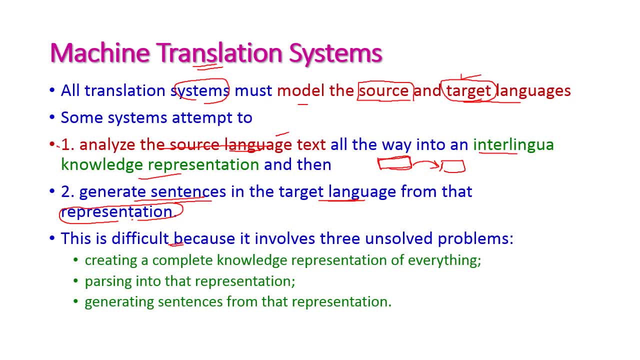 And this process is very difficult because there are three unsolved problems. First one is creating a complete knowledge representation of everything, And second one is parsing into that representation And third one, generating sentence from that representation. So these three are unsolvable problem. Why? Because the grammar rules of one language will be completely different to grammar rules of another language. 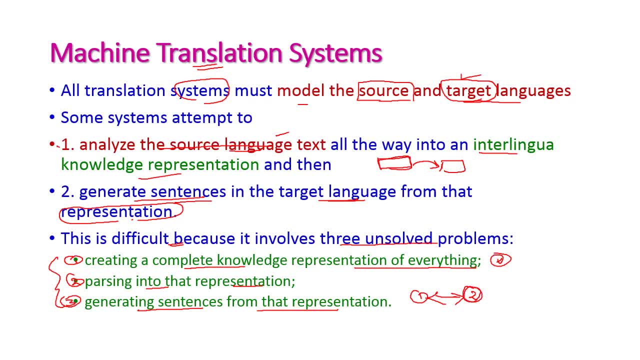 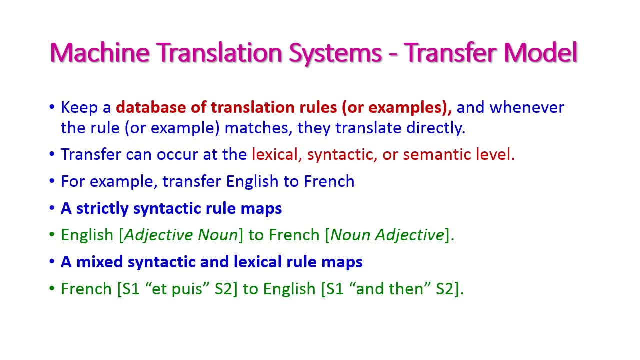 The target language, the other language, because both are natural languages and the natural language grammar are completely different. The transfer model of machine translation system. So this transfer model keeps a database of translation rule or examples. So the translation rule is nothing but the grammar rule. 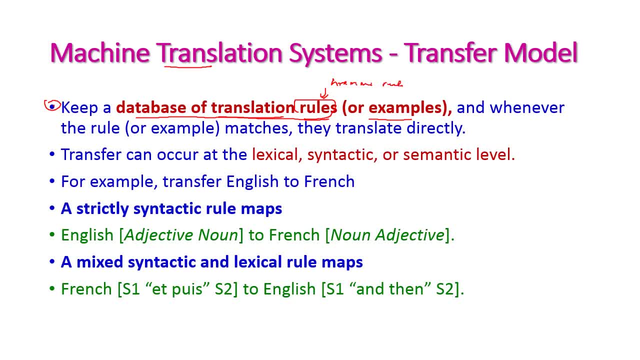 Grammar rule of that natural language, and whenever the rule is not there, the translation rule is not there. So the translation rule is not there, So the translation rule is not there. So whenever the rule matches, they translate directly. That means whenever the rule matches from one natural language to another natural language, then the translation will be taken place. Okay. 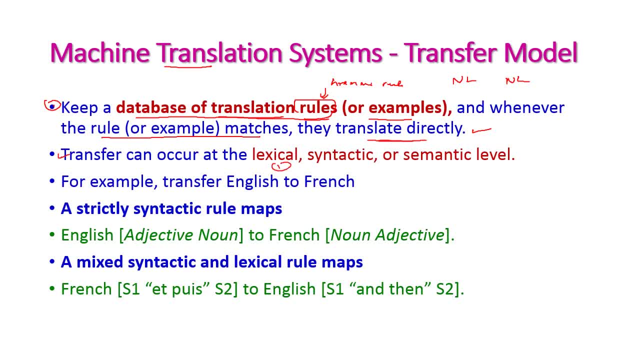 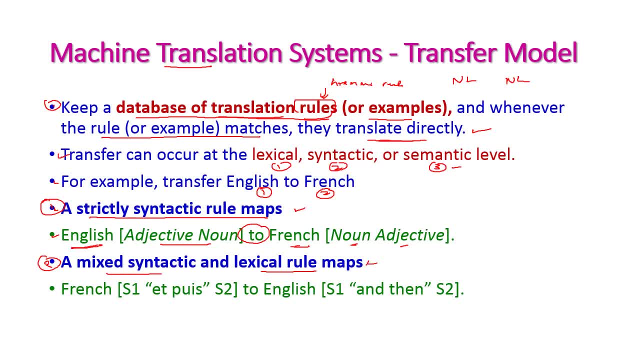 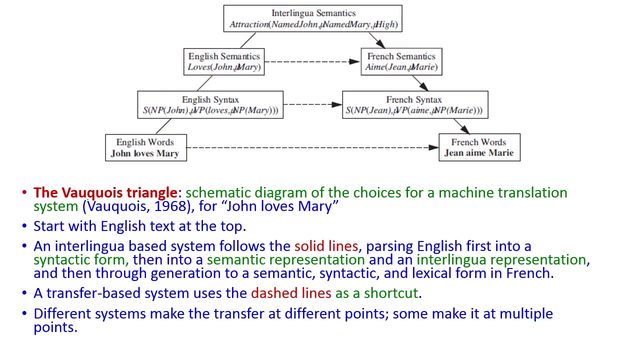 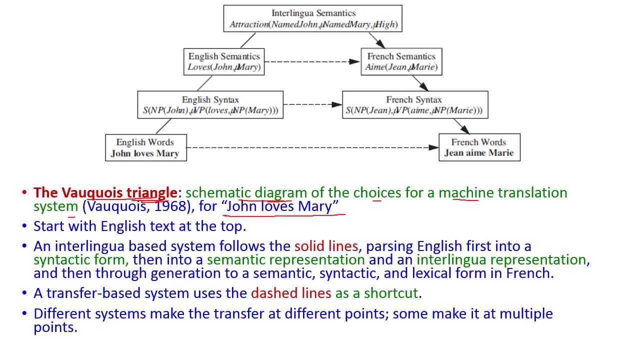 system for the given sentence: john loves mary. this is a english sentence. right here the system starts with the english text on the top, so the system starts here. first step: okay, the given english word is john loves mary and the second one, the interlingual based system, follows solid. 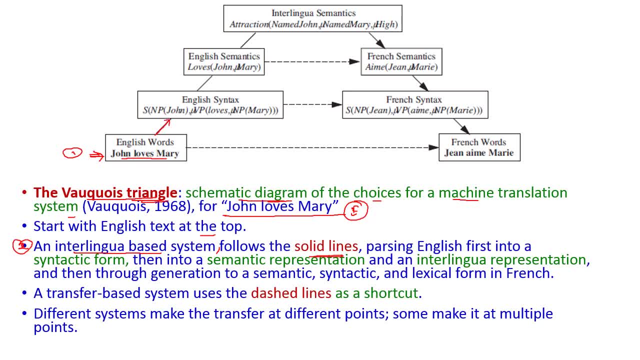 line: okay, see, this follows the solid line. okay, the words will given to syntax and syntax will given to english. semantic: okay, and this is interlingual semantic right. so the interlingual based system follows the solid line, passing english into a syntactic form and then semantic. 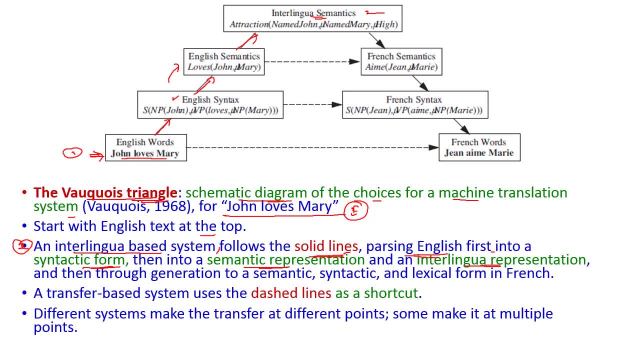 representation, after that interlingual representation. okay, this is the second stage, third stage and fourth stage. okay, after that, ah, the generation to semantic, syntactic and lexical form in french. okay, so, after interlingual semantics, that will be converted into french semantic, after that french syntax and then french words and finally we will get french word. okay, so, 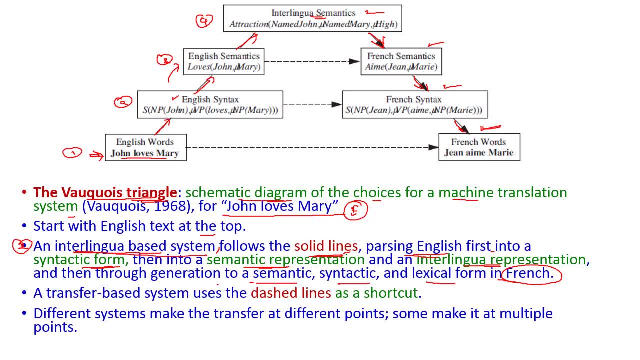 this is interlingual based system and this and the transfer based system use the dashed line as shortcut. okay, so the dashed line represent the equivalent of english words to french word, the equivalent syntax, english syntax to french syntax, and english semantic to french, his semantic. so this is the shortcut. 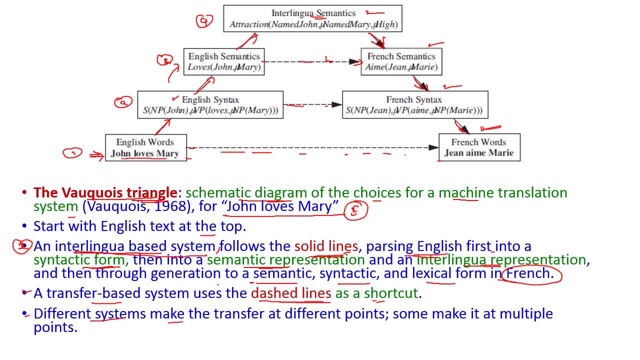 way. okay, but the different system makes, ah, different transfer points and some make multiple points. that is what they refer, but we will well see to demonstrate later. okay, the difference system. uh, i ii some sense. uh, if i add two into one, we will see that again. the difference system. 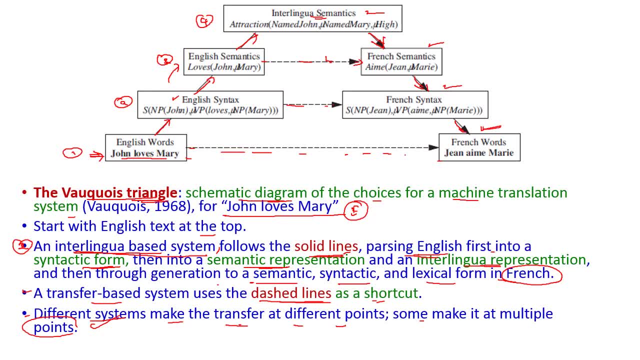 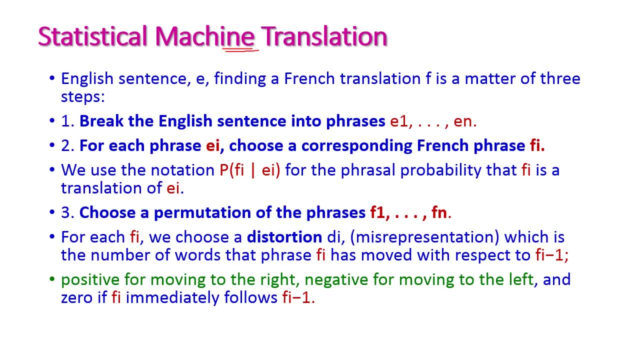 goes here괠 s our DIY: very making simple, multiple points also, so some of the language may have multiple stages. the statistical machine translation: okay, here the English sentence e. finding the French translation F is the matter of three steps. okay, the first step: break the English sentence into phrases, that is, e, 1, e, 2, e, n, etc. up to e, n. that is the. 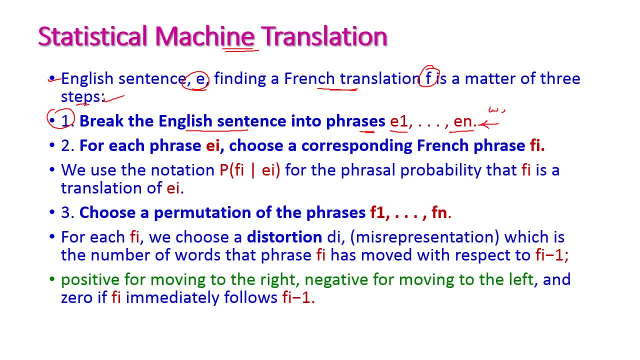 sentence will be braked into number of words. if it is English words, then it will called as e 1, that is small e 1 and second one for each phrase: e. I choose the corresponding French phrase. okay, for each phrase, the corresponding French phrase will be selected. okay, so the notation used for this translation: P F. 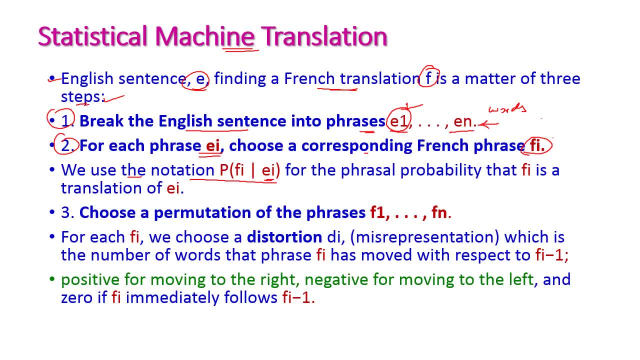 F I, such that e I, that is, e I, will be translated into F Y. okay. and the third one is: choose the permutation of phrases F 1 to F n. okay, for each F? I we have to choose distortion di, that is, misrepresentation, which is the number of words that phrase. 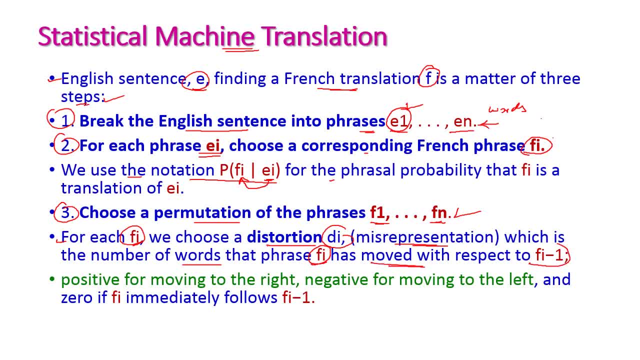 F I has moved with respect to F I minus 1. okay, why? because the English words, when translated of words, are passed on side by side and this behaviour will get loving right. as E, F, F so is described. whatever translation means, the grammar of French is different from the two used in agreement. right, according so. 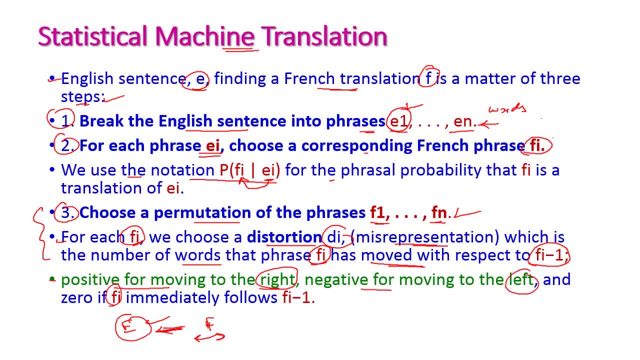 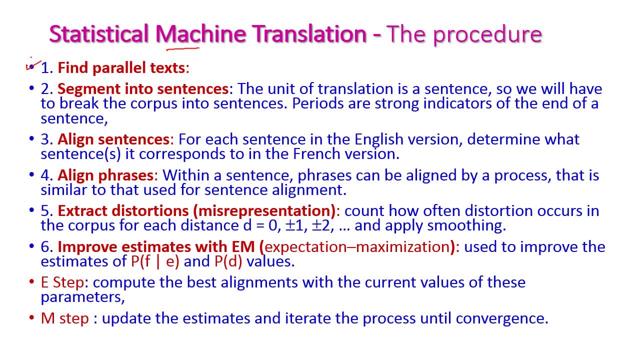 the grammar of F. that translation, OKa, is the traduction, French word again. the grammar will not be the same anymore. that is the specifications of F, F, y. the first step: find the parallel text, parallel text of English to French, okay, and second, one segment into sentences: okay, that is the entire, very big statement. that is sentence will be. 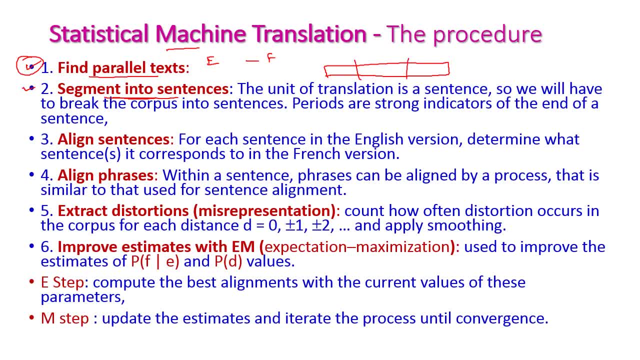 divided into small segments. okay, the segment is not a single word. okay, it may be a group of words. and third one is Allen sentences, that is, for each English version determined what sentence correspond to French version, so this is called as Allen sentence. and fourth one is Allen phrases. 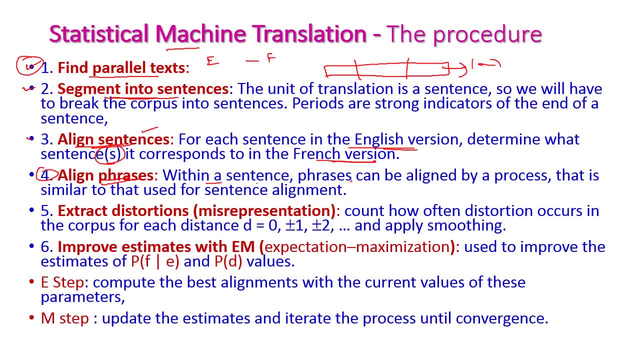 that is, for each English phrase we have to find the corresponding French phrase. so this is Allen phrases. and fifth one is extract distortion. distortion means misrepresentation. okay, here we have to count how often distortion occurs in a corpus. corpus means a complete sentence for each distance, d equal to 1, sorry, 0 plus or minus 1, plus or minus 2, etc. okay, and apply. 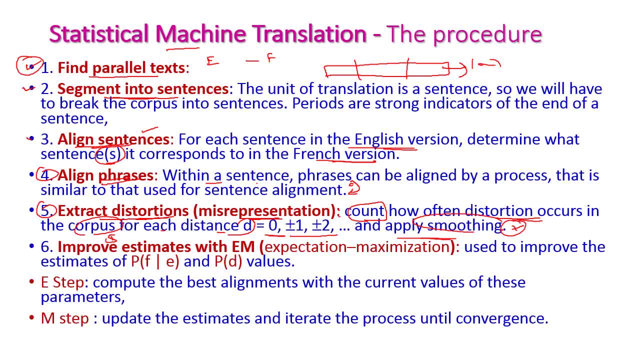 smoothing right. destruction means in what way the sentence will be shifted, either from left hand side or right hand side. how many words will be shifted? okay, and the sixth one is improve estimates with em. em means expectation and maximization algorithm. this is a popular machine learning algorithm which is used to improve the estimates. 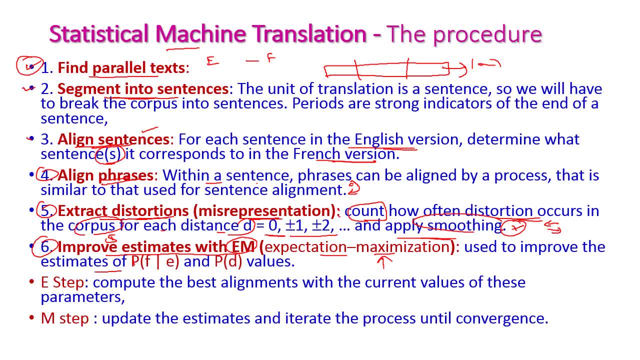 of ah, pf f, such that E okay- and pf d values right. pfd means the distortions and when come to E step, it computes the best and the bad state of distortion that we have to do right. so to this, we need to alignment with current values of those parameters and when come to m step, it update estimates and 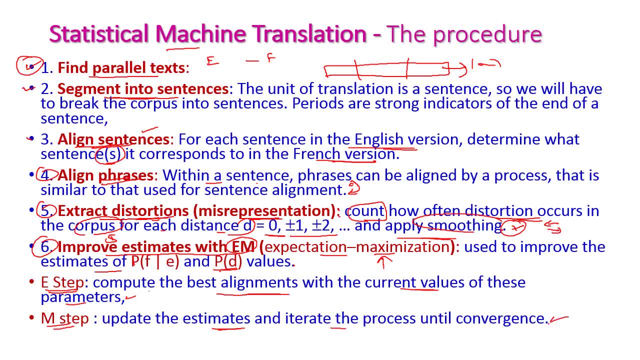 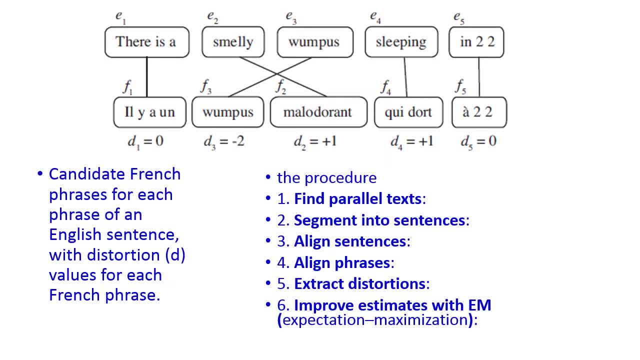 iterate the process until it converges. okay, let us see all those things with one example. so this diagram explains the english sentence: there is a smelly bumpers sleeping in two, two. okay, the equivalent french sentence is given like this: okay, so consider the french phrase for each phrase of an english sentence, with distortion d values for each french phrase. 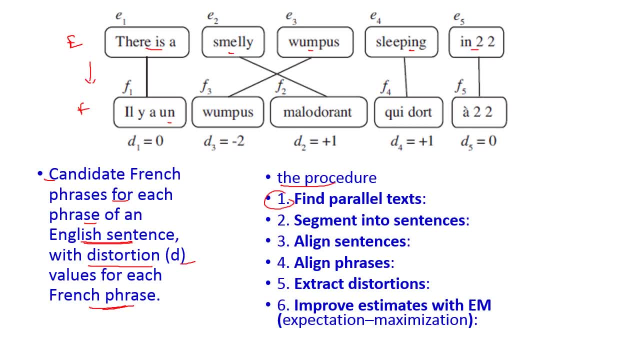 okay, so now let us see the procedure. first one: find the parallel text. so these are the parallel text, okay, the parallel text for each english word to french word. and second, one segment into segment sentences. So segment: the complete sentence will be divided into 5 different segments. ok, The 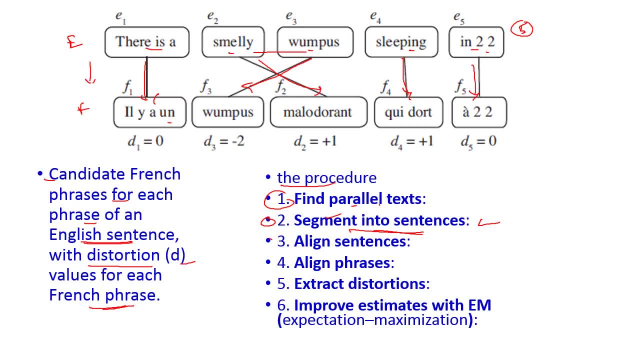 complete sentence will be divided into 5 segments. and third one, Allen sentence. So Allen sentence means we have to find the equivalent sentence in the French, So this English language to French language and Allen phrases is also the same. and fifth one: extract, distortions, Extract. 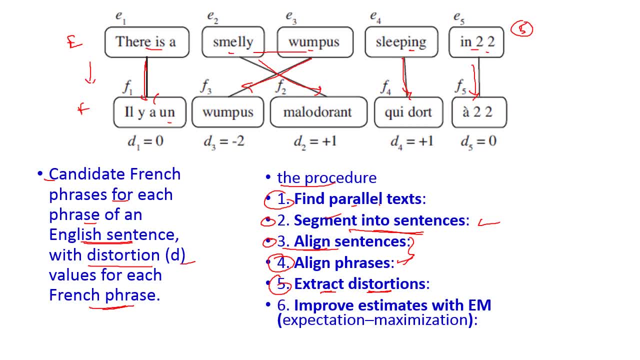 distortion means how the sentence will be deviated. So there is here, there is no deviation. but when come to smelly bumpers, this will be deviated. First noun will come, after that adjective will come. ok, So that is in French format. So this is, ah. the interchange will be.